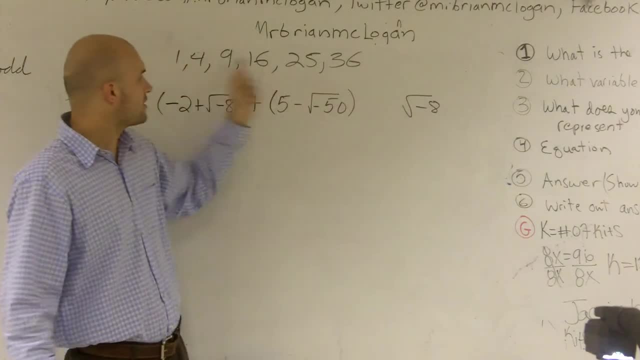 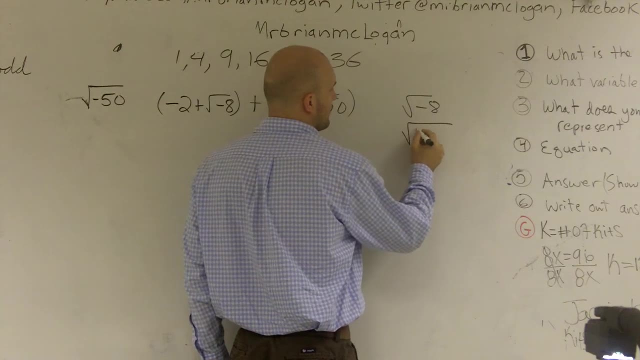 Well, here I know I can take the square root of 4, and it also goes in the square root of negative 8.. So what I'm going to do is I'm going to rewrite this as 4 times a negative 2,. all right, 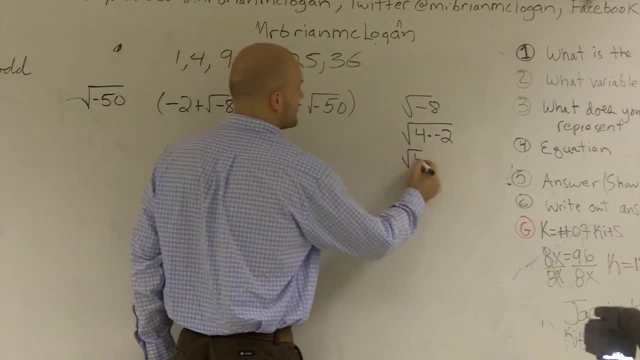 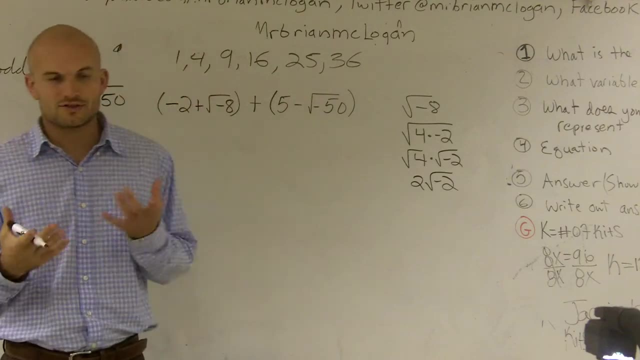 And now I can break this up and do the square root of 4.. Square root of negative 2.. Square root of 4 is 2. Square root of negative 2.. Now you still can't. there's no two numbers that multiply to give you a negative 2.. 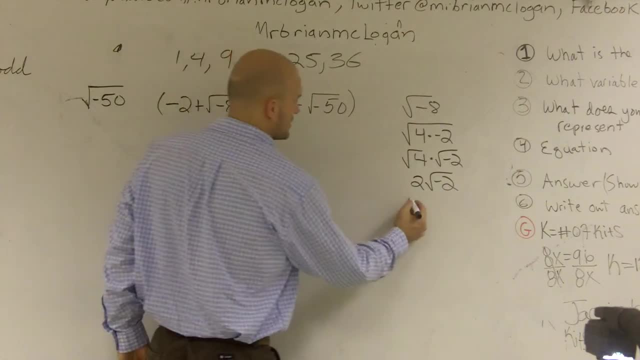 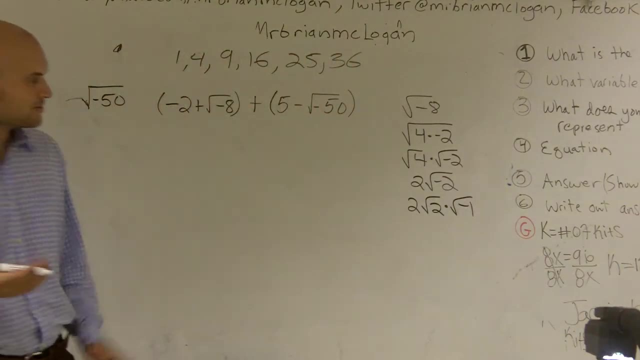 So what you're going to want to do is we need to say: well, let's break this up and do 2 square root of 2 times the square root of negative 1.. All right, Because negative 1 times 2 is going to give you negative 1.. 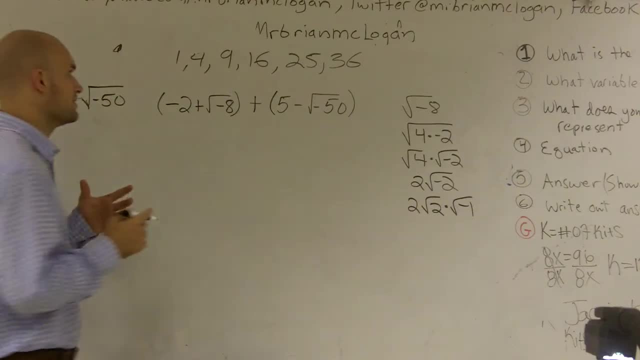 And one thing you guys should know about this is: what is the square root of negative 1?? Well, that's what we call in complex numbers, i. So if I can rewrite this, If I can rewrite this as negative i, what this really is is 2 times square root of 2 times i. 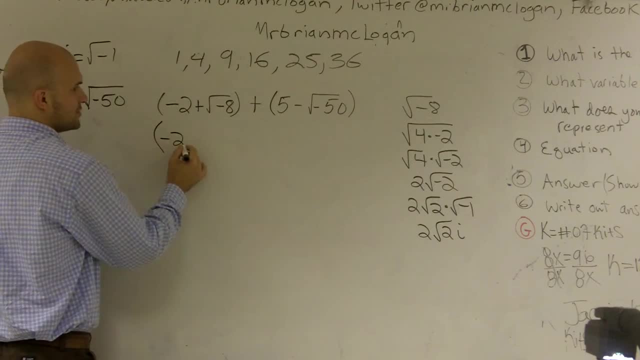 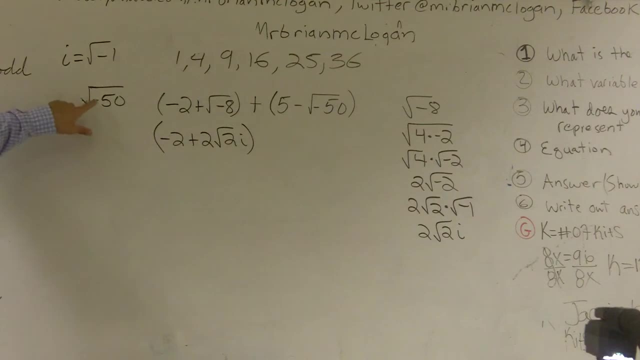 So let's now. I can probably rewrite square root of negative 8 as negative 2 plus 2 square root of 2i. Now let's go and look at 50.. 50, since it's negative, I can factor out my negative 1.. 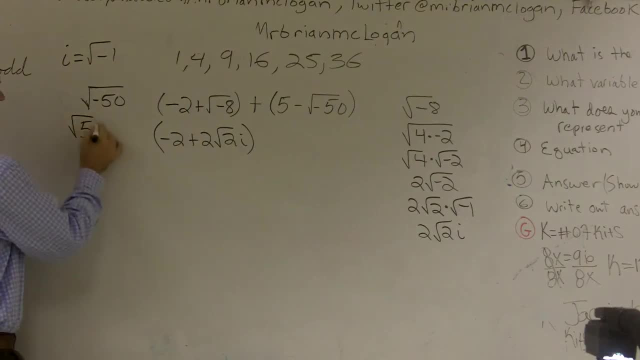 So really, this is going to look like a square root of 50 times a negative 1, which would really be square root Of 50 times i. Then what square number goes into 50?? Well, I can rewrite this as square root of 25 times 4.. 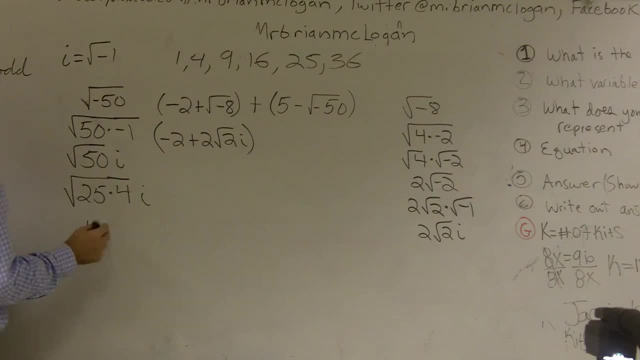 And then i at the end. The square root of 25 is 5.. I'm sorry That's 2,, isn't it? Square root of 25 is going to be 5 times 2i. So plus 5 minus. 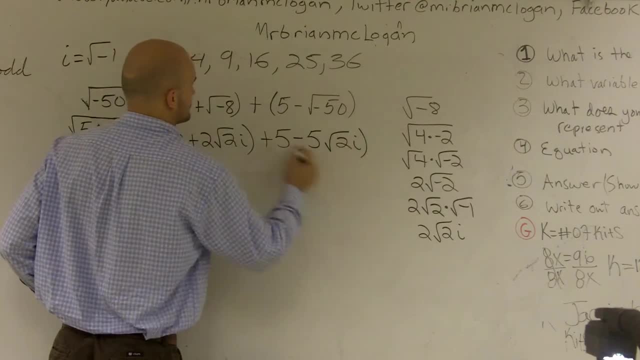 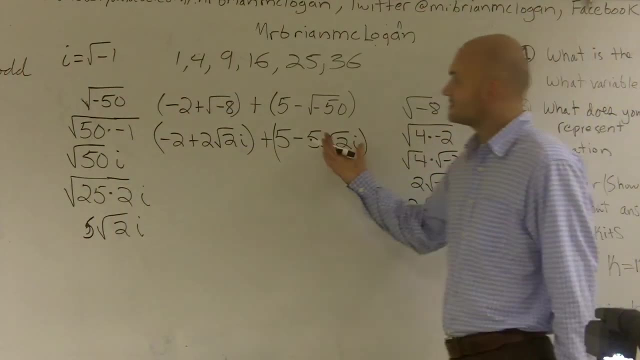 5 times the square root of 2i. All right, So now that we have this all set up, so now what I've done is I've simplified my radicals, And now what I need to do is I need to add them. 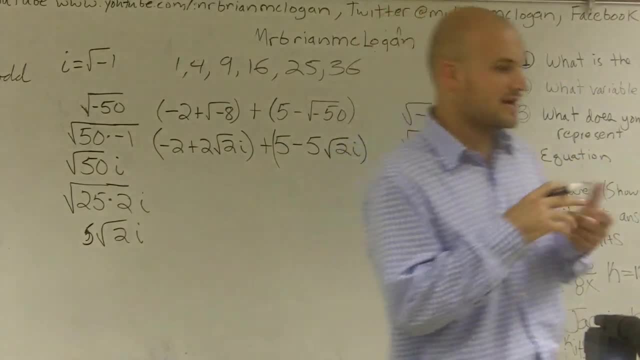 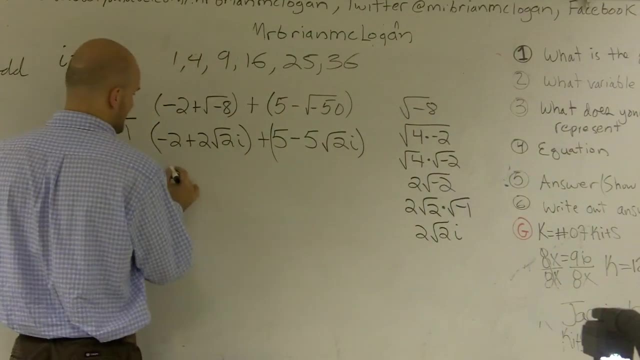 So the main important thing when adding radicals is we need to make sure that you can only add the real components and the imaginary components. So when we're looking at complex numbers, we have this is a plus bi, And this one would be c plus di.